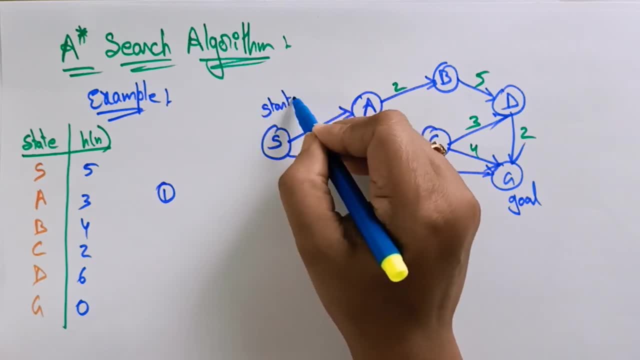 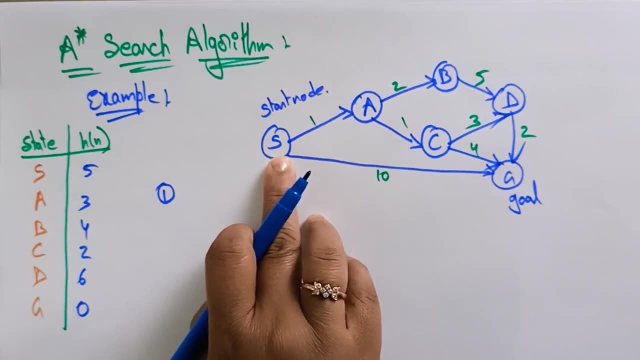 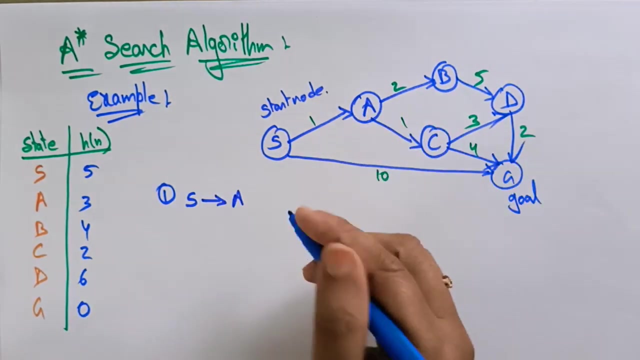 So start, this is a start node. Let's take this is a start node, Start node From starting. first start node: what are the two successors for S, A and G? Okay, So let's take S to A. Let me take first this path: S to A, S to A. what is the F of n? F of n is equal to G of n plus H of n. We know the formula. So G of n is the cost from that start node to that particular node. whatever we are calculating, 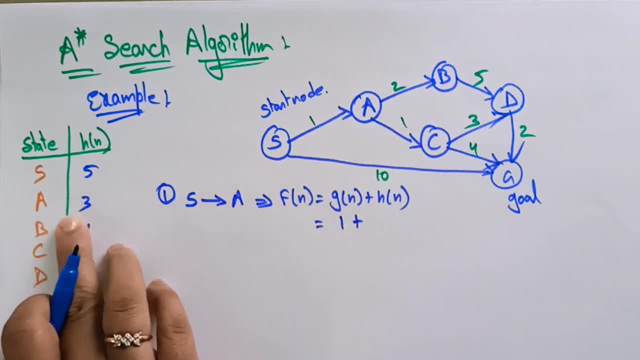 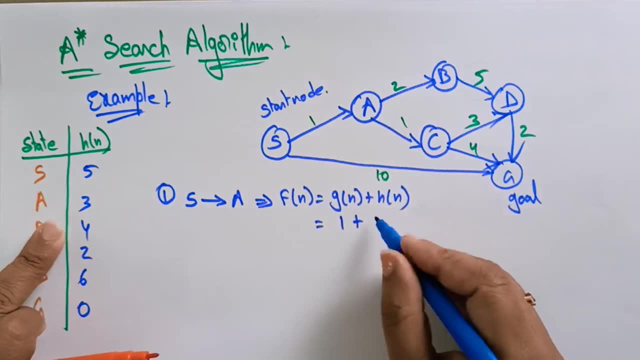 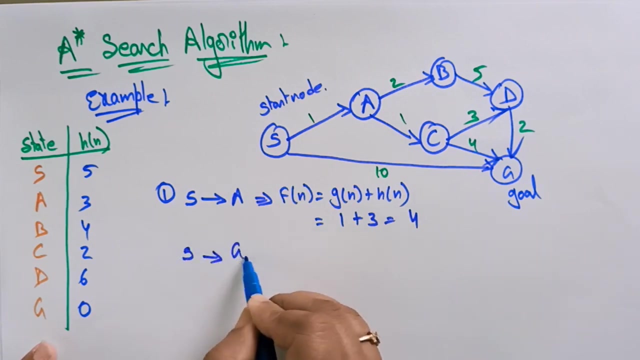 Here it is 1.. And A heuristic value is: we are going to this node, So you need to calculate the heuristic. You have to take the this value. Heuristic value of A is 3.. So you got 4.. So this is 1.. And again, here S goes to G. also, The starting node has two successors, So S goes to G. So what is the F of n? G of n is 10.. And H of n for G is: 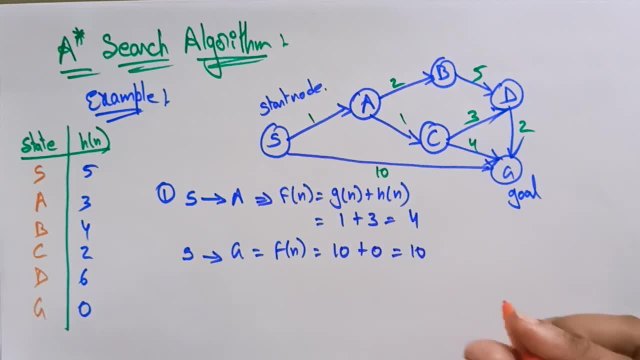 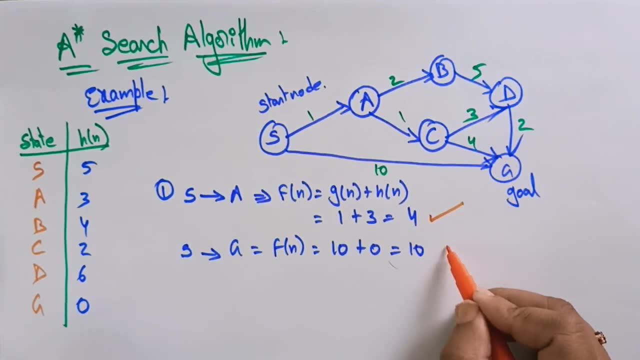 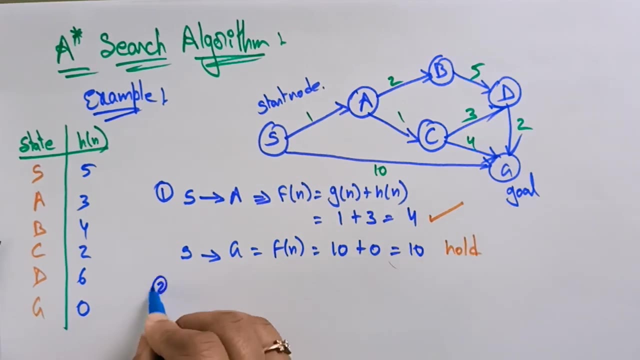 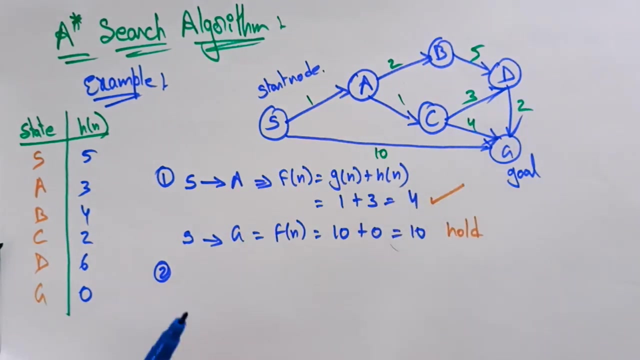 0.. So you got 10.. Which one is the best means the lowest heuristic value. So obviously this is low. So you just keep this as whole, Keep it in whole, Don't remove it, Just keep it in whole. In the next step we need to check which value is less. So next, coming to this A, So I am taking this path because I just kept this as in whole. I just kept this path in whole. Now I am taking this path. So A. what are the successors for S? 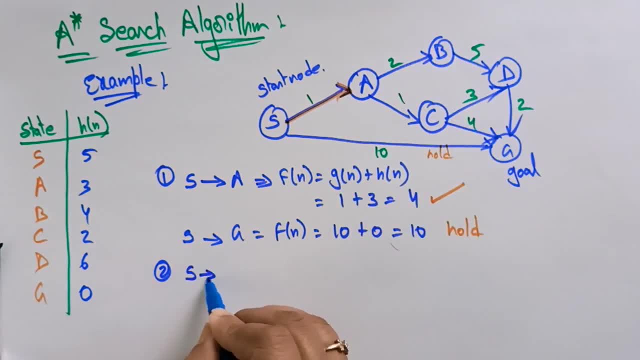 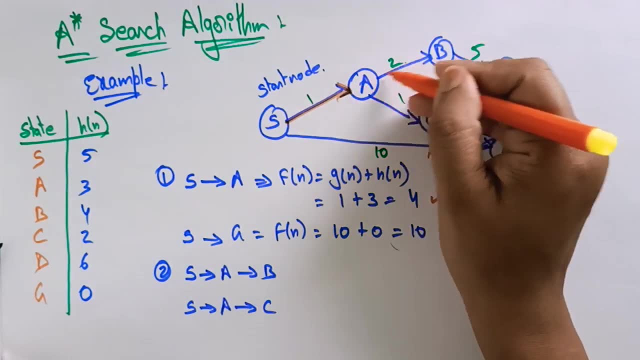 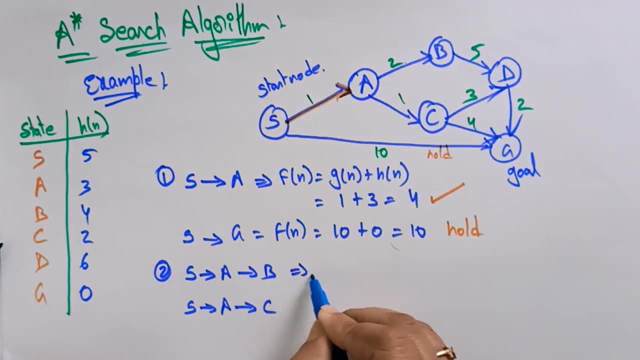 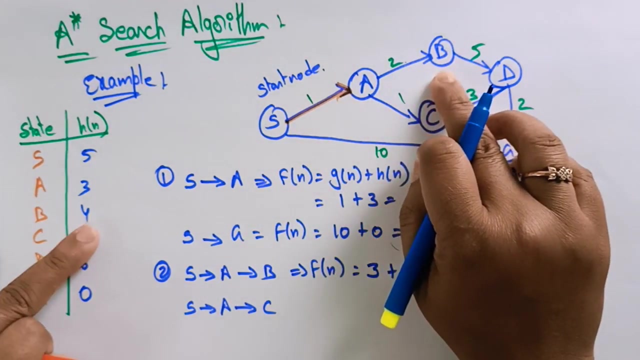 Successors of A, B and C. So S A B and S A C. So there are two paths. are there S A B and S is A to C? So which one is the best? I need to be checked. Now calculate F of n, F of n. G of n is 1 plus 2.. That is a- 3.. And what is the heuristic value of B? Heuristic value of B is 4.. 3 plus 4, 7. I got Now calculate. 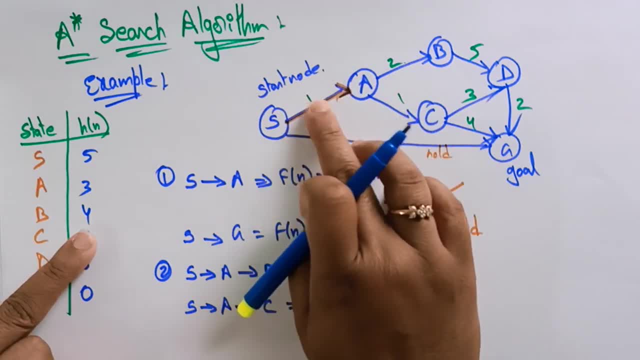 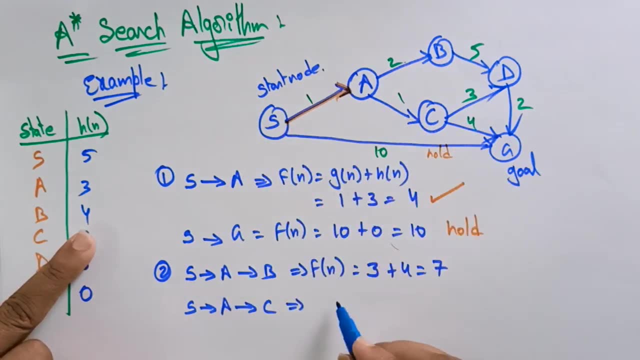 first Remember this: S, A, C, G of n is 1 plus 1.. Okay, The cost of that node, from starting node, 1 plus 1 is the G of n, That is, 2.. And what is the heuristic value of C, 2.. So 2 plus 2, 4.. Which one is the best? Obviously, here, this is the best. Okay, Here, this is there, and this is there, and you just keep this as in whole. Okay, From this to anyone you can select. Either you can select. 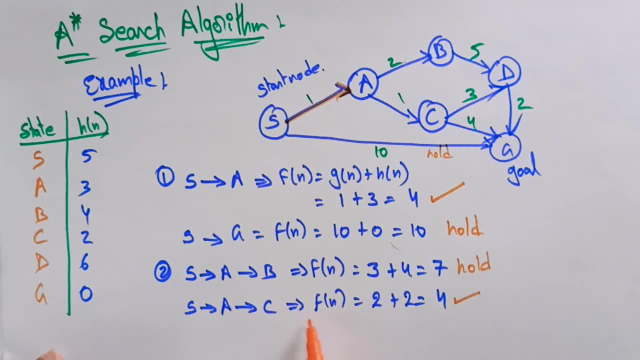 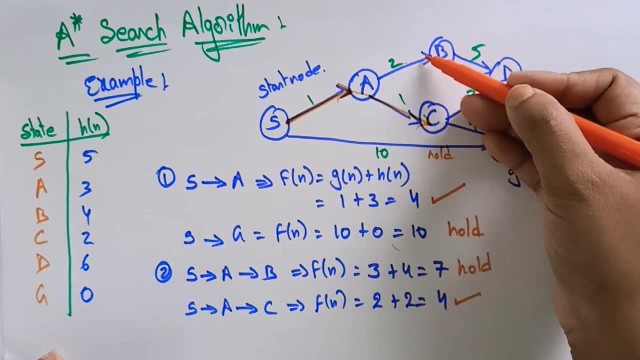 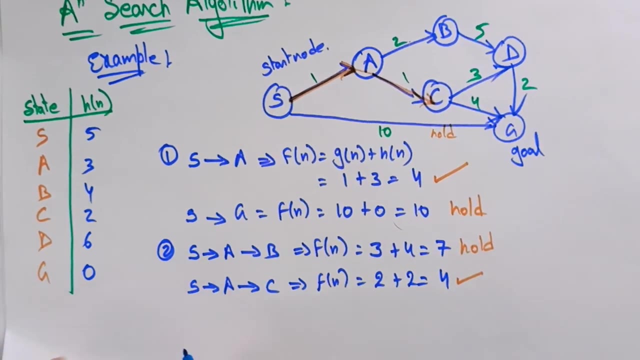 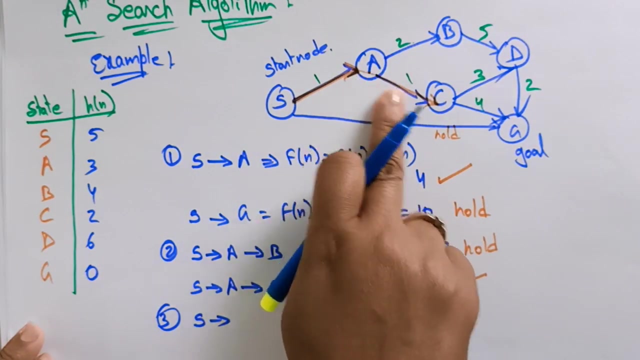 this is the best: S determines A to C. This path is I selected. Okay, Rather than this, I am selecting this path because it is 7, you got More value, got, So just you keep that. it in whole, Okay Now 4.. And the third step: So from here, Yes, So here, S to A, I already selected. So S to A to C. So from C, you are having. 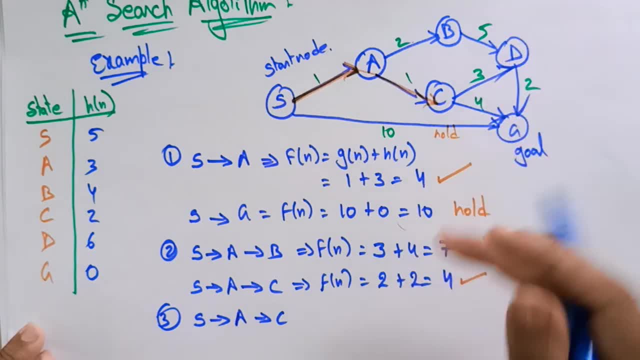 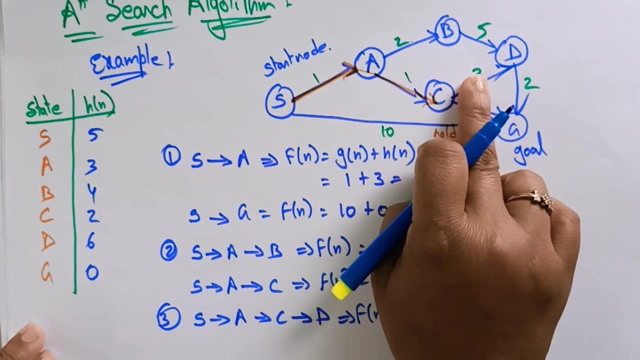 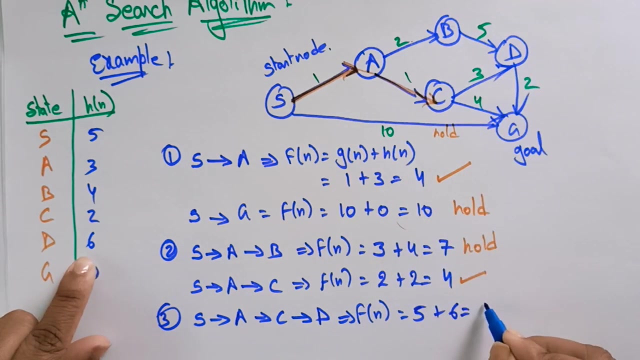 2. 2 nodes. One is G and another is going to D. So first let me take S to A, A to C. C is going to D. So what is the F of n value for this? You need to calculate the cost: 1 plus 1,, 2.. 2 plus 3,, 5.. And what is the heuristic value of D, 6.? So you got 11.. And another path. What is another path? S, A, C. 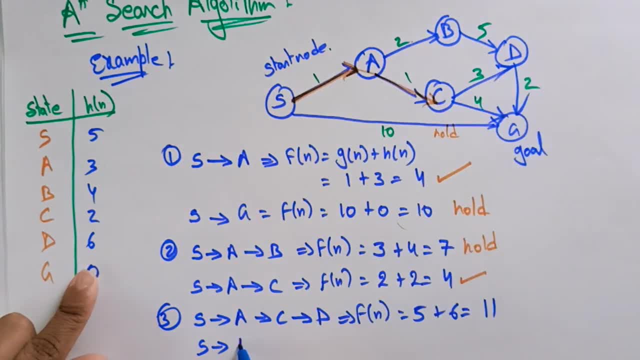 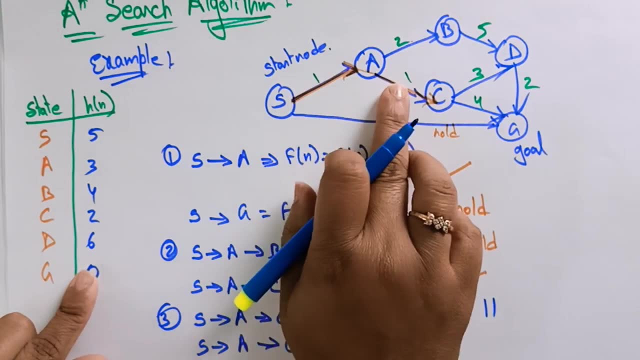 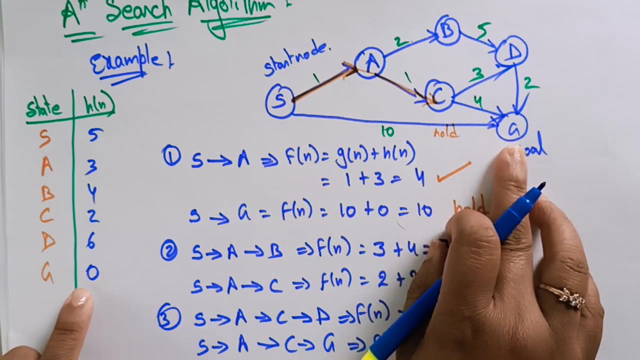 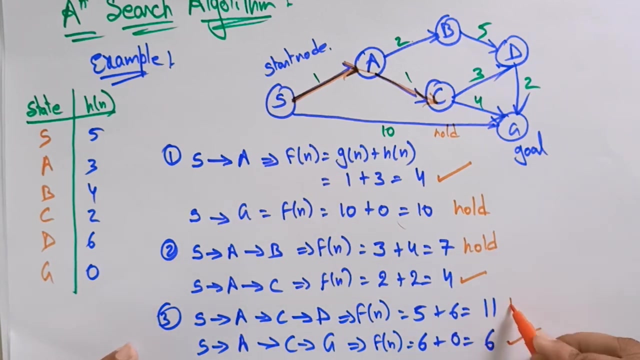 G, is there D? I calculated S, A, C, This time G. What is the function G of n value is 1 plus 1, 2.. 2 plus 4,, 6.. And what is the heuristic value of G, 0., 6.. So which one is the best? Obviously 6 is the best And I am keeping this whole. So why I am keeping? So now check this 6, this value to the.